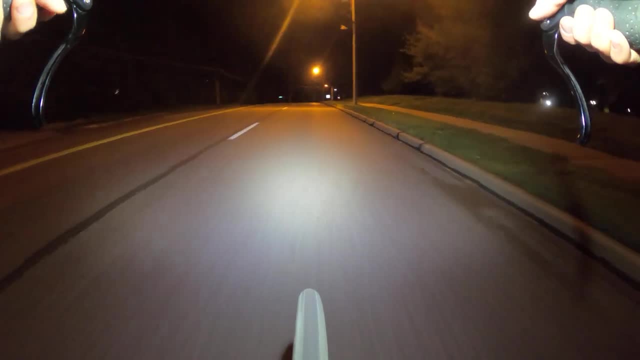 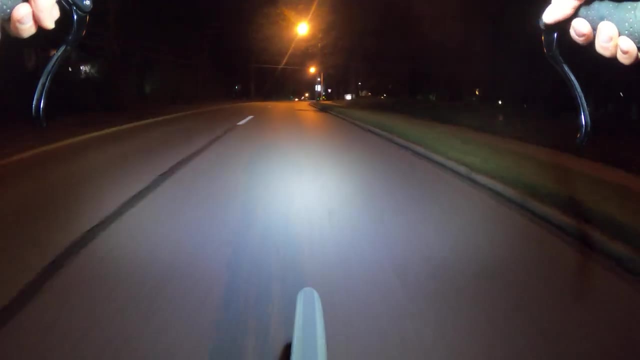 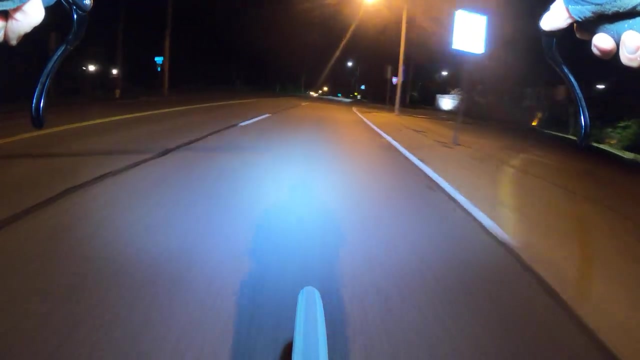 100 PSI into it, Maybe more. And by really skinny I mean a tire that's only like 25 millimeters wide or 1 inch wide. Woo Made up the hill. Um, if it's a little wider of a tire, like on a. 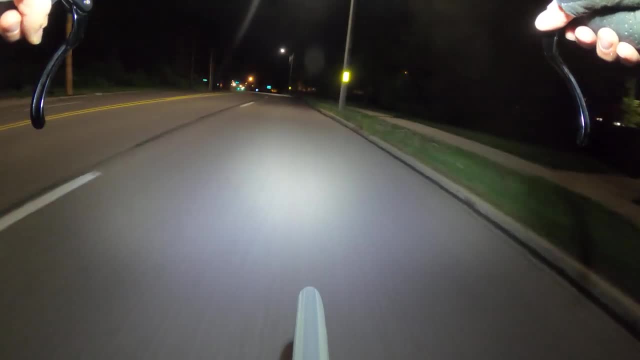 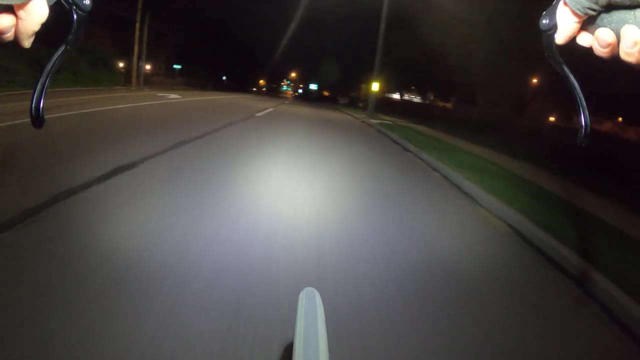 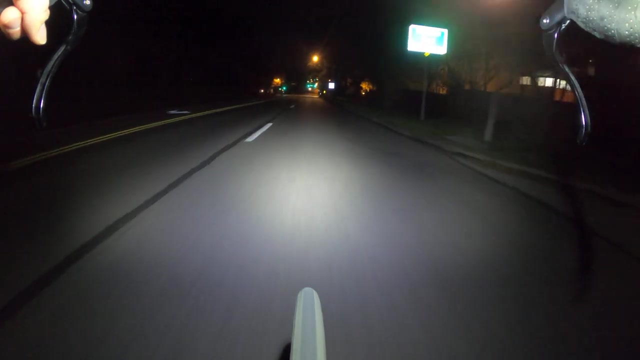 on a gravel bike, adventure bike, cyclocross bike. you want to aim for at least 80 PSI. Could take it up to 100, though I wouldn't worry too much about over-inflating, but you definitely don't want to under-inflate. 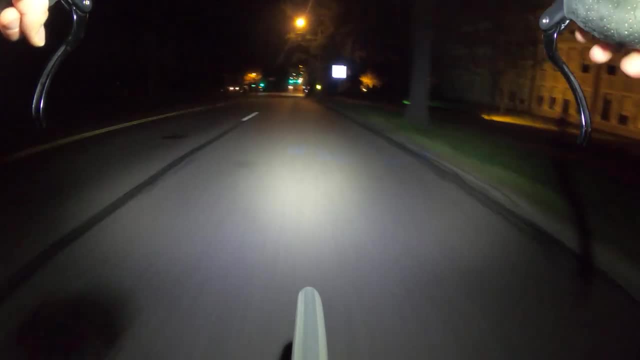 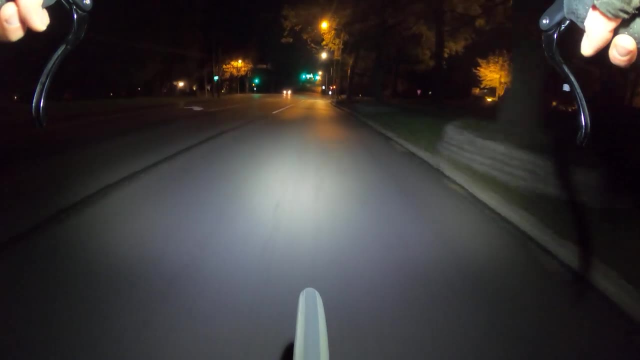 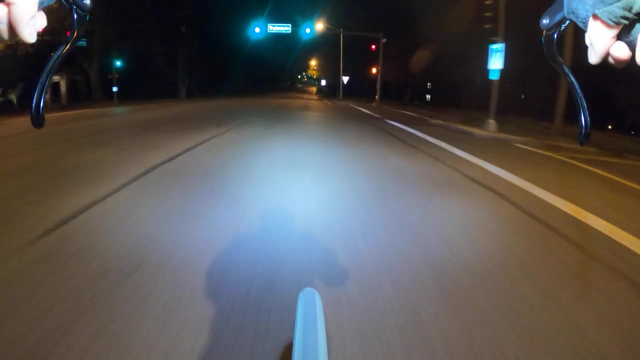 under-inflate, because you risk yourself getting a puncture. That is where you get a flat tire. So that brings me to knowing how to change a flat tire or a basically a punctured inner tube, Because chances are, you're probably not riding. 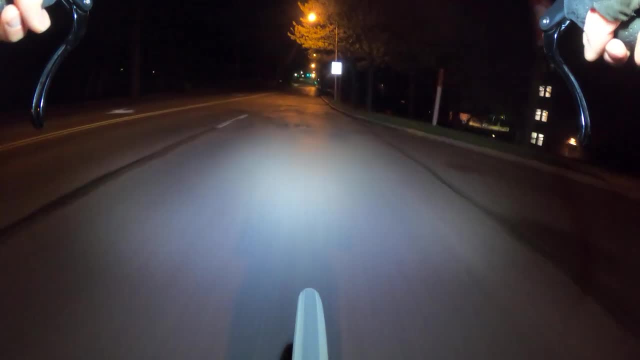 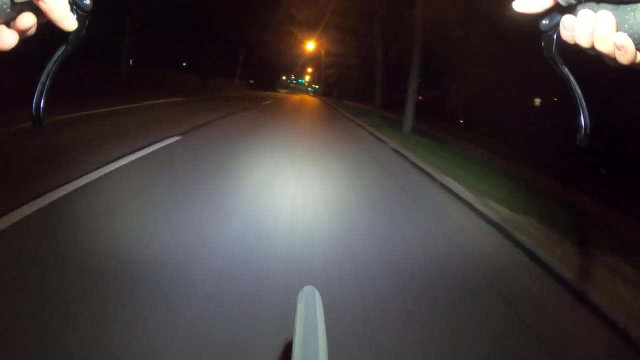 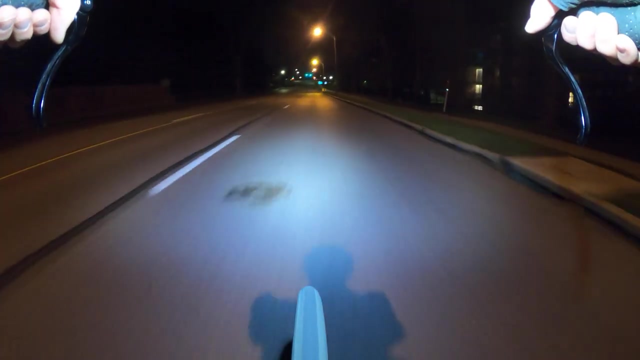 uh, you know, without an inner tube. It depends if you have a mountain bike. A lot of mountain bikes wheel rims are meant for, uh, without that inner tube. But anyway, what is B? B is brakes. You got to make sure the brakes are working well. 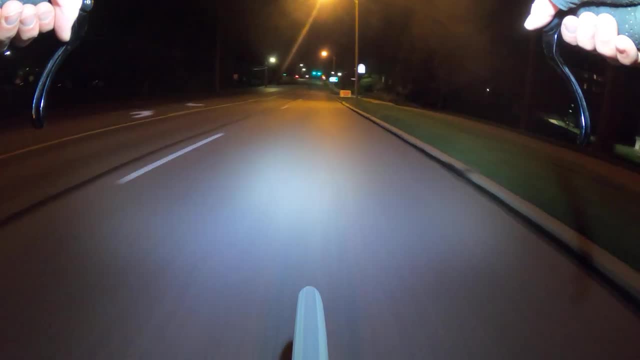 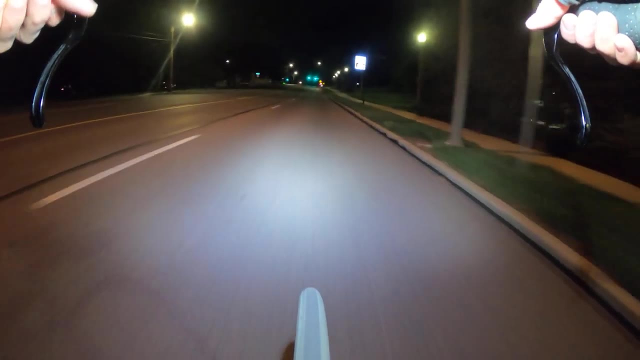 Brakes are very important, So pretty self-explanatory. but know how your brakes work, Know if there's something jammed. If there's something jamming them up, You know how to fix it or you have the tools to fix it with. 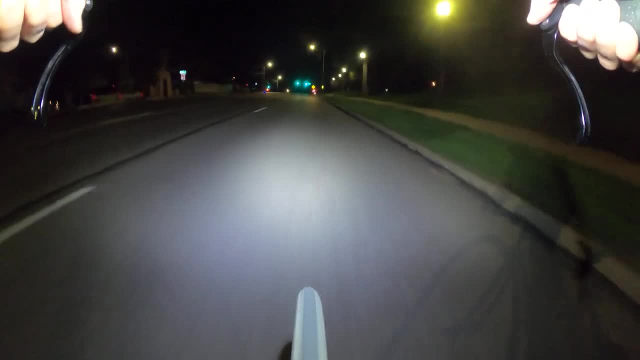 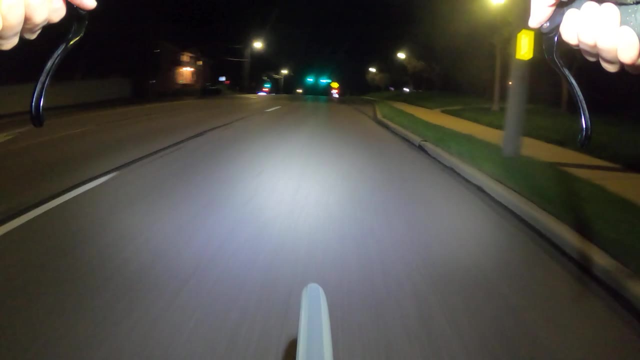 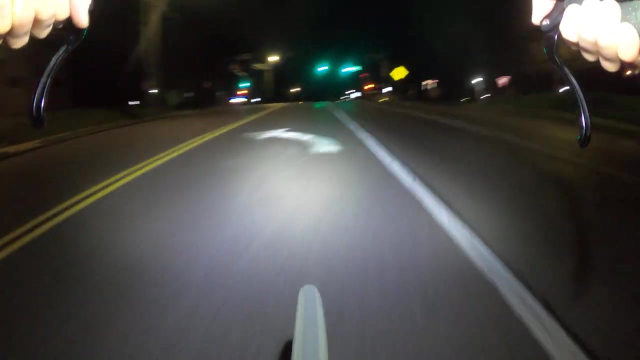 Typically, all you need is like: uh, an Allen wrench, basically Typically a five millimeter wide or a four millimeter Allen wrench. Let's go to the left here. Whoo Up, Up there. Whoo Hang a left here. 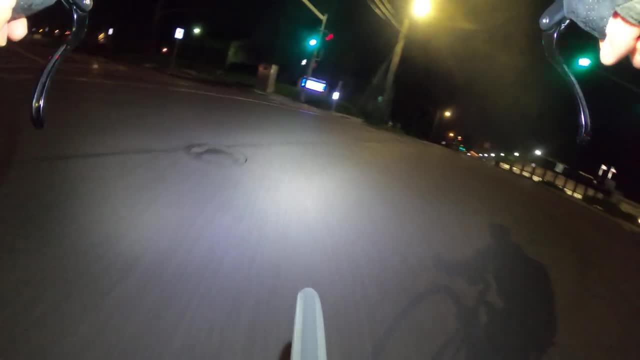 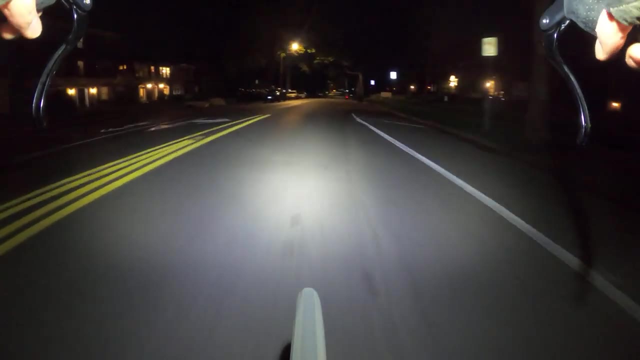 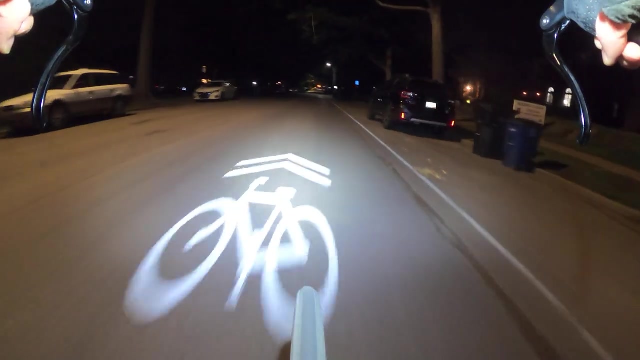 On our way. On our way, Whoo, Whoo, Even though it's really chilly. the one benefit is I'm not really sweating too much As long as I'm not too overdressed Whoo. So yeah, that's B for brakes. 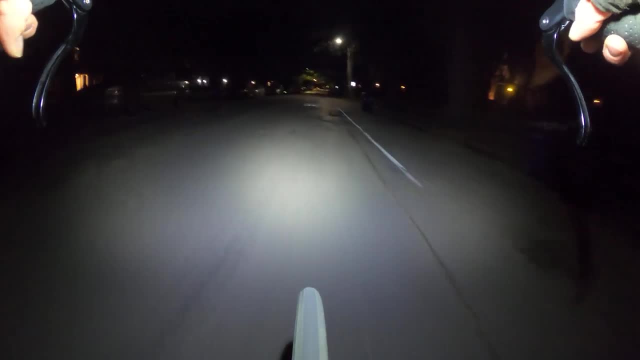 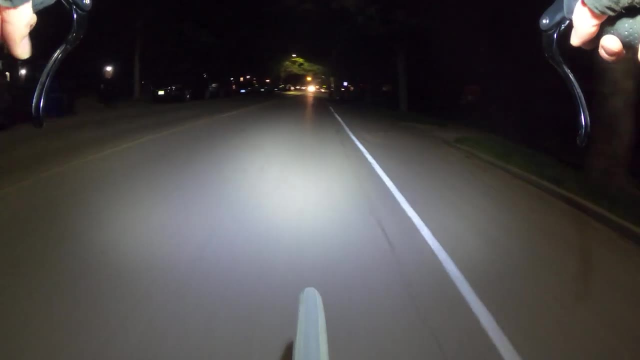 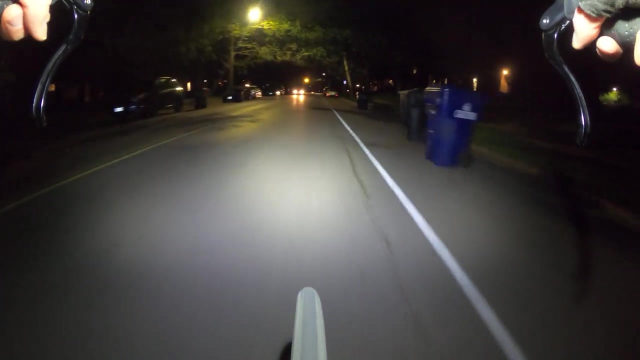 Now, what is C? C is the chain or cassette, Basically the drive train on the bike. So you want to keep that well oiled. There's a couple of different types of chain. there's a chain oil. You can even put a kind of a chain grease on there. 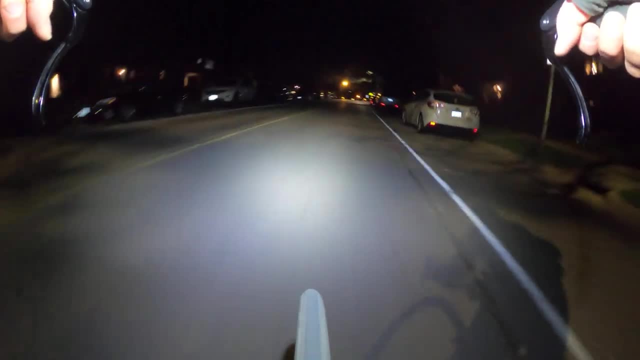 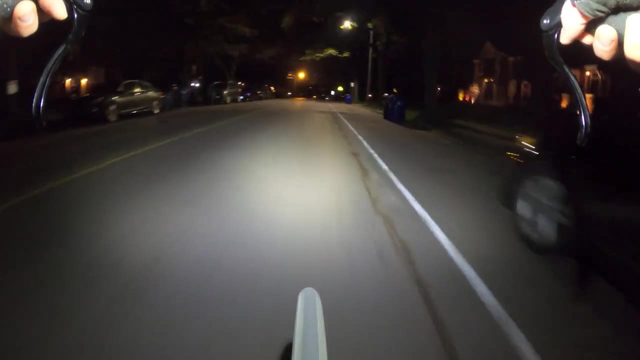 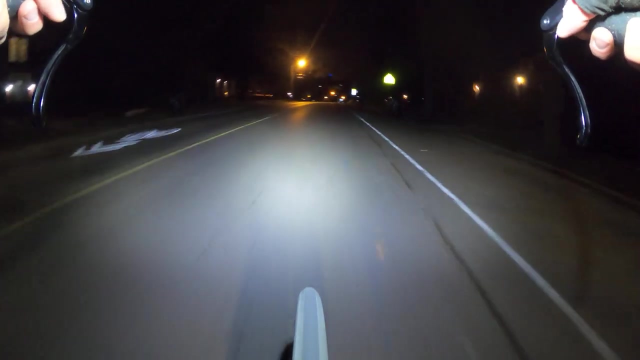 which can last longer, although it can gather a lot of gunk over time. So, yeah, I would recommend oiling your chain probably once a week. You know, I mean, I do less than that honestly, But yeah, probably once a week isn't that bad. 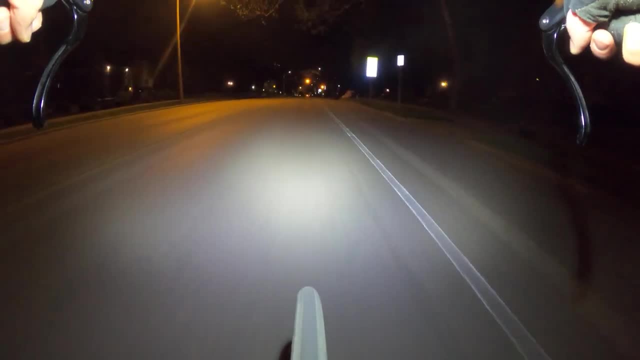 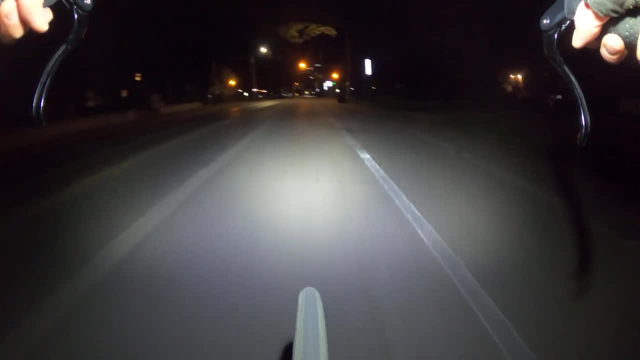 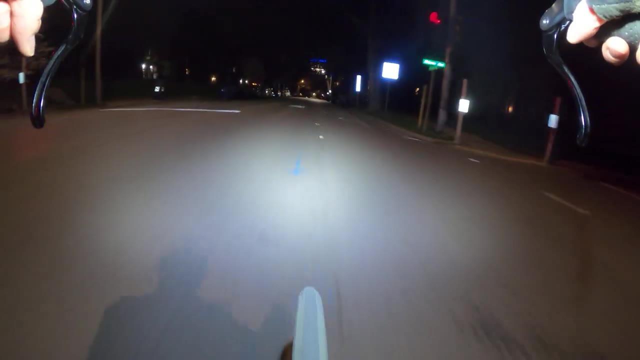 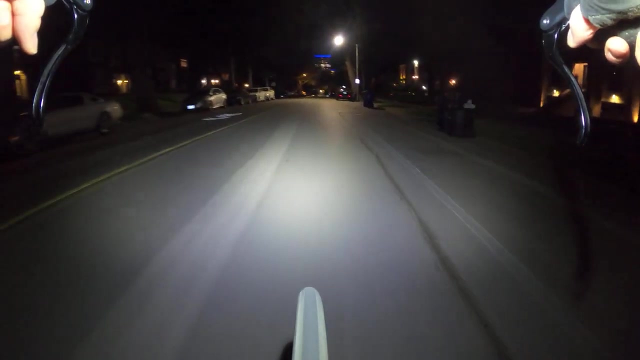 And it will get into all the little crevices. You get really particular about it and get it. you know, one drop on each link. I don't think you need to worry about it to that extent. Whoo Adi-dad-a-da. 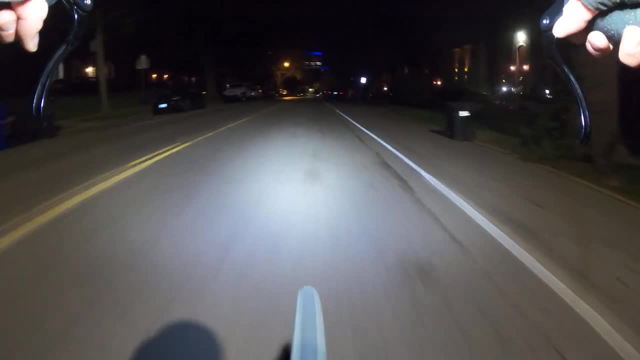 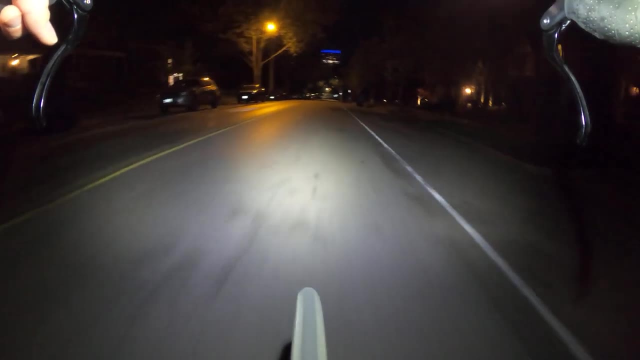 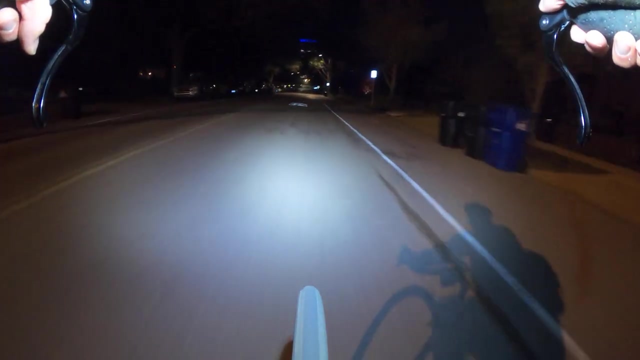 Oh, no, Sounds ABC. Oh yeah, The cassette, right, Well, that's the cog. I guess the chain ring and cassette. Those are the sprockets in the front and the back of the drive train. Really the best way to clean those. 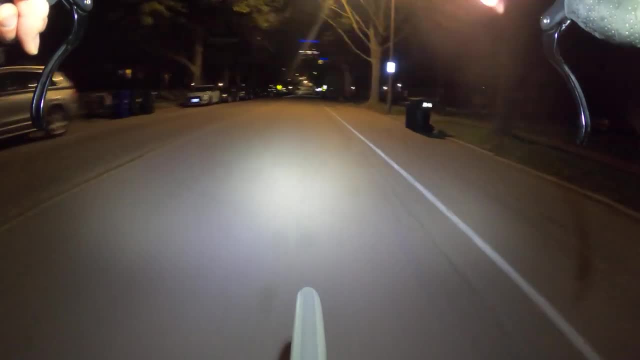 is you gotta kinda take the chain off pretty much, cause getting those teeth cleaned are kind of difficult. So I guess C could stand for clean- keep a nice clean. So I guess C could stand for clean- keep a nice clean. So I guess C could stand for clean- keep a nice clean. 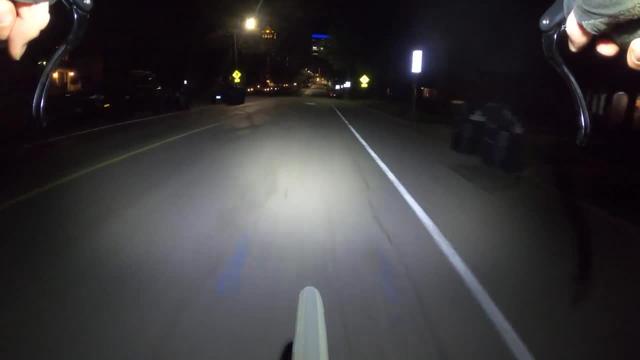 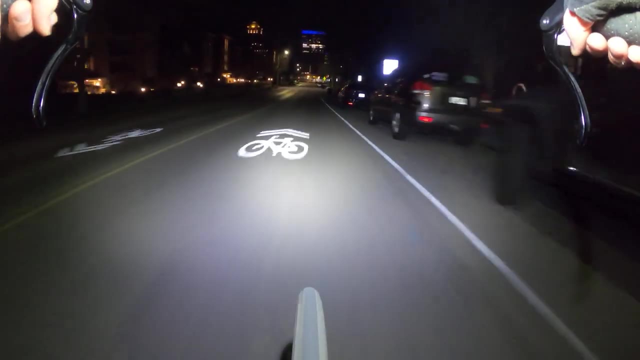 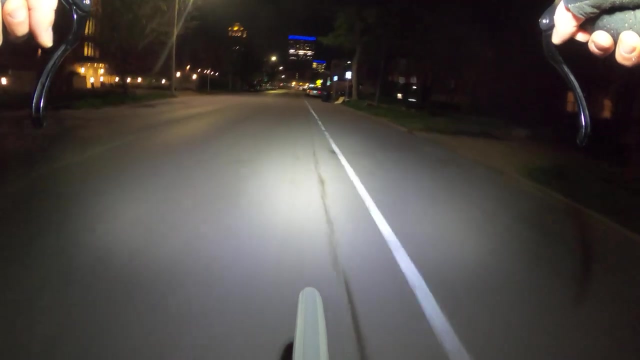 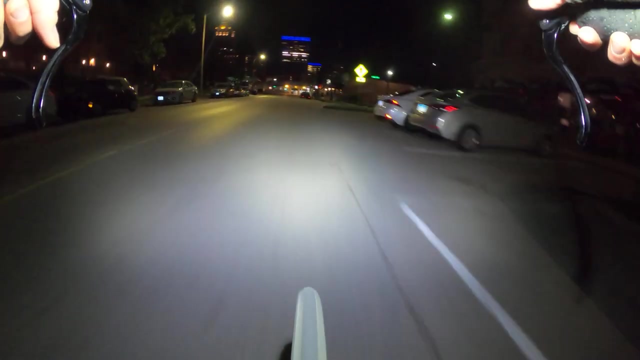 bike. so another thing is when you're about to head out in the morning, very simply you can check all these things: check your quick release, see if the lever is disengaged or partially disengaged, and then ABC, check the end of tires. you know, squeeze the tire, bounce the bike. you'll be able to know right. 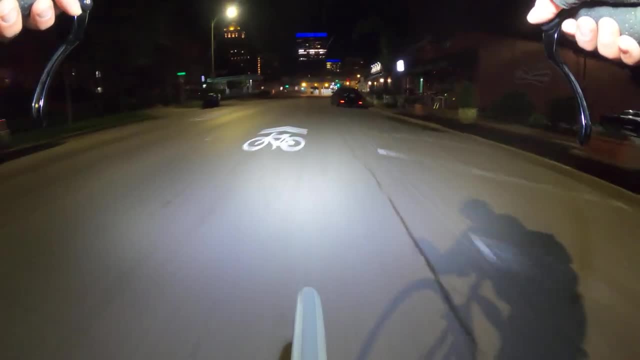 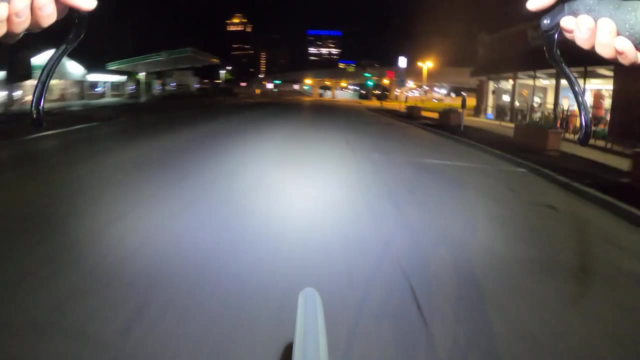 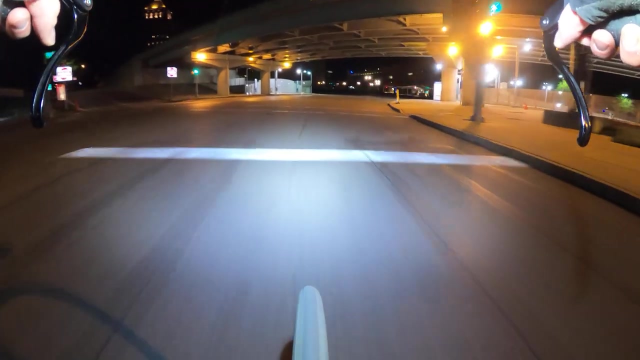 away if it's really deflated, which can happen sometimes. if you have a really slow leak overnight, they can just lose all the air. another reason: I also suggest pumping up your tires before you head out there in the day. if you got a bike pump at work, that also helps. 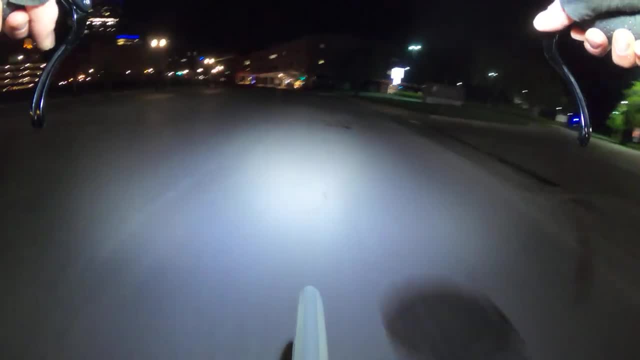 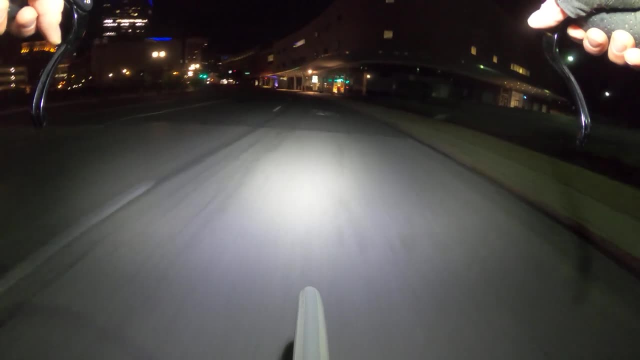 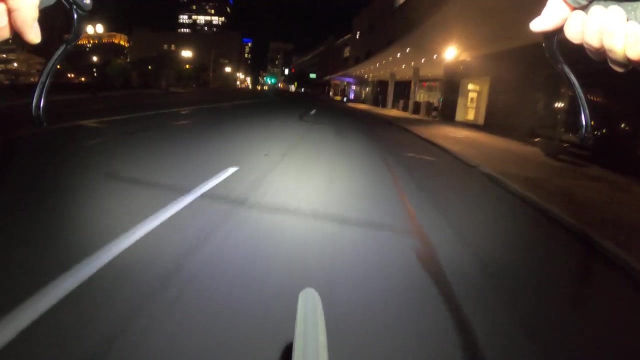 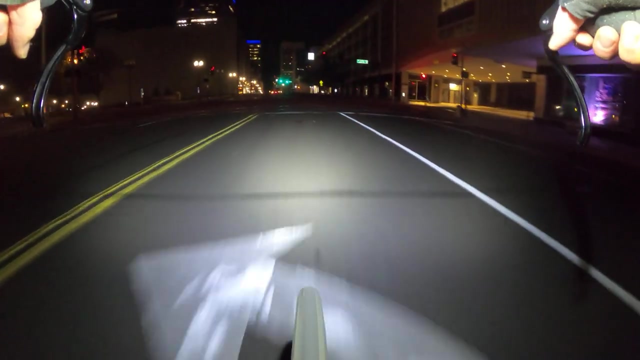 into the city and then brakes. you know, just squeeze your brake levers before you get on the bike. make sure the brakes are actually engaging when you roll the bike forward. nobody around. we'll go this way. actually, there's nobody around, so let's go this way. 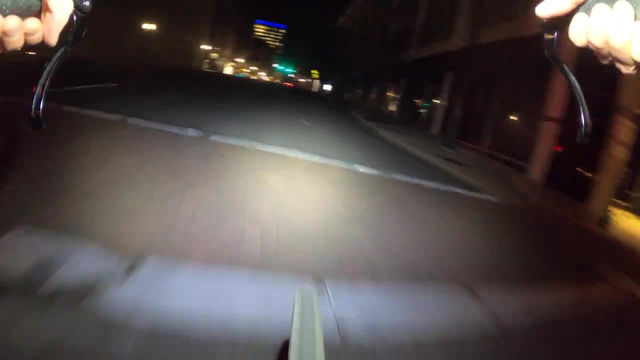 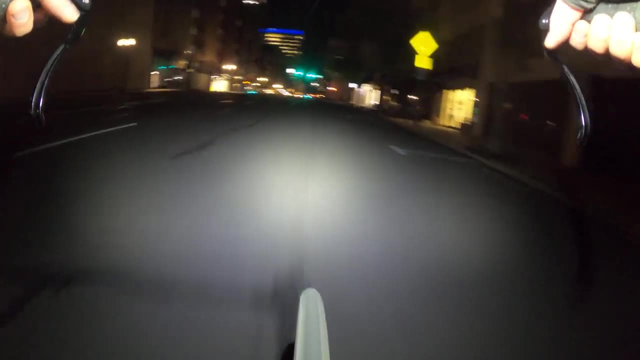 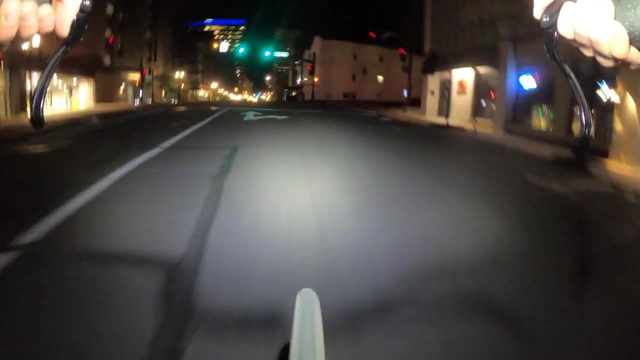 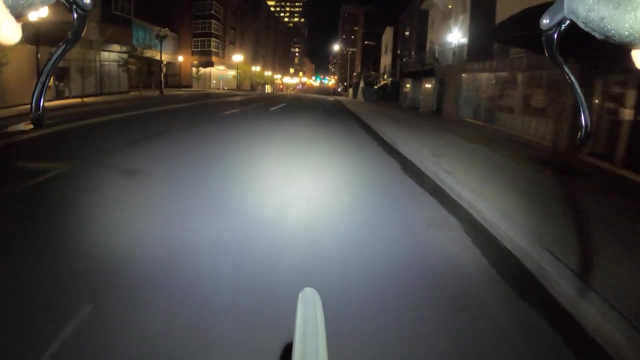 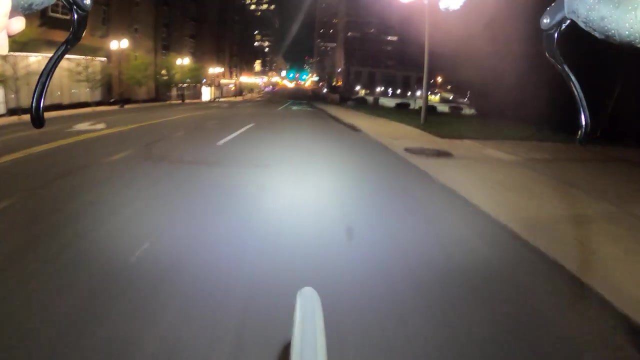 normally I wouldn't jump across lanes like that. this is the only way we can bean past this. I have a feeling this light up here that's green will stay green for us as long as it's not out of traffic. whew, and then for the chain, you know, just kind of spin the spin the the pedals you. 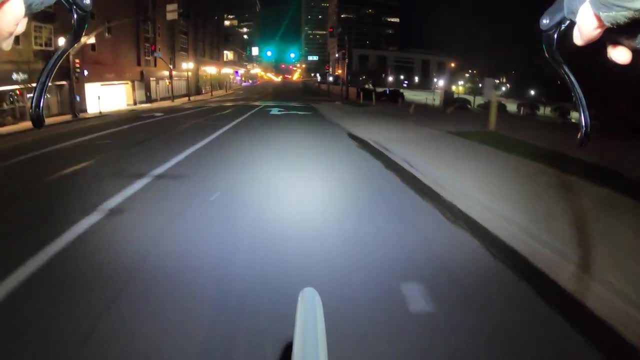 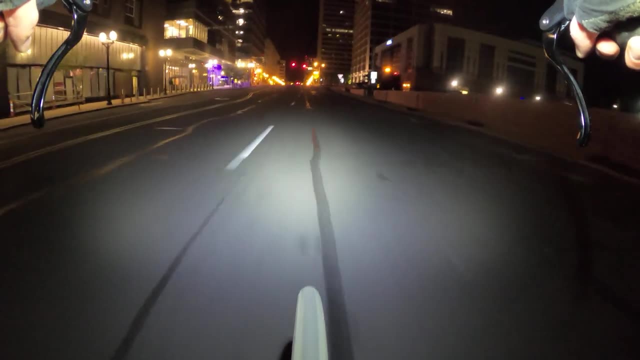 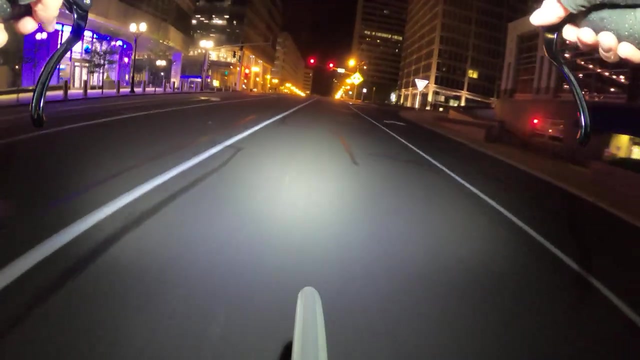 know backwards. make sure the chains not just falling off- is gonna get, is gonna get just falling off or something. bounce the bike. make sure there's nothing wrong with the drivetrain- pretty much, but uh, especially check the air and the tires and then the brakes. if you're only going. 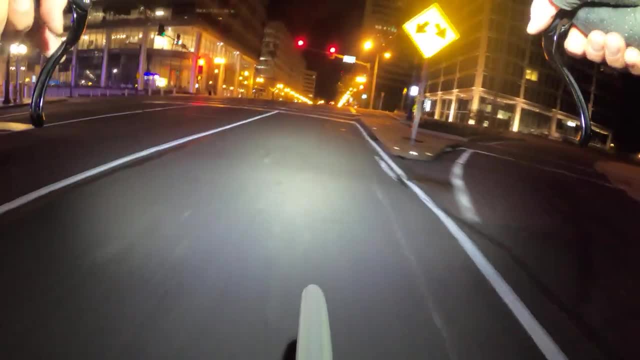 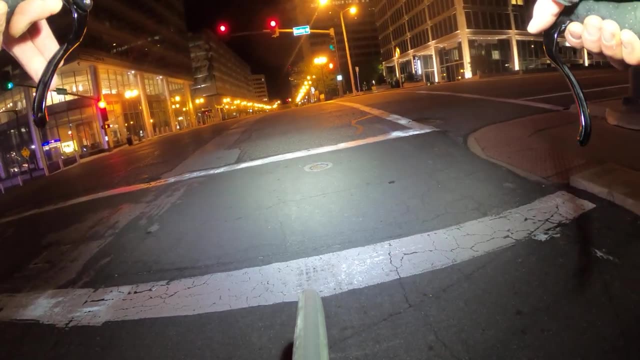 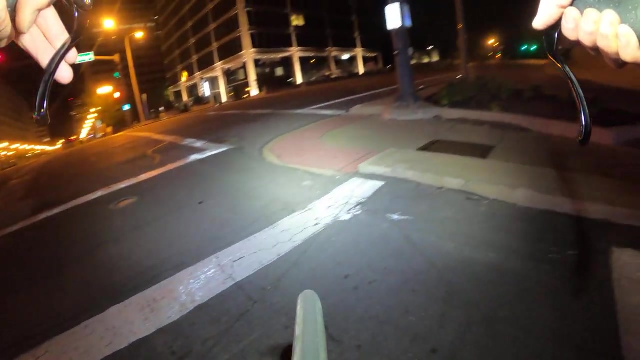 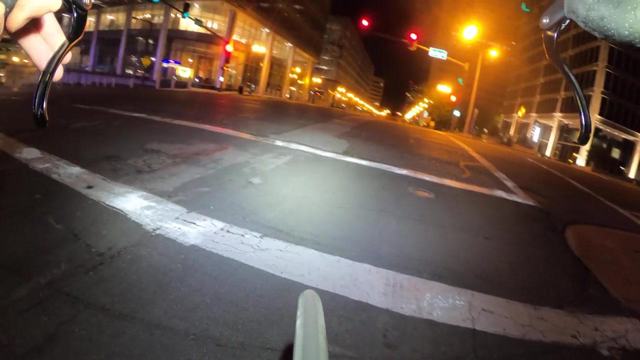 to check a couple things. bounce the bike, squeeze the brake levers. you're probably pretty good to go um. the uh, the light over there is buzzing or something. i was wondering like what the heck is that sound? sounds like my uh three wheel, my bike. i don't know if this light's gonna work for us here. 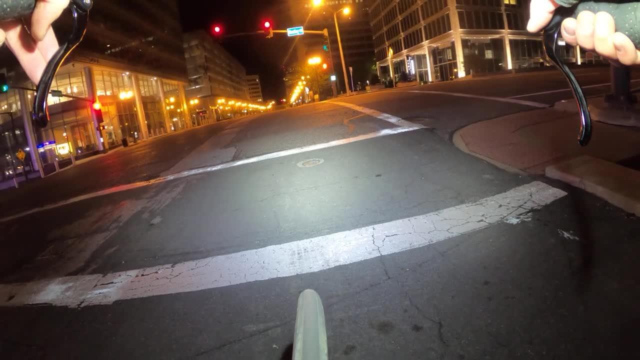 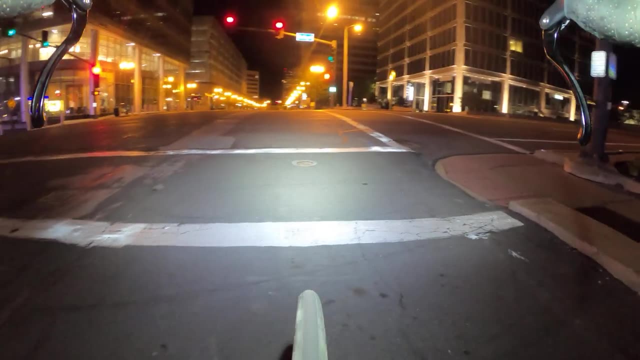 see it's like it says don't walk, like it's gonna stop. it's not changing. and i got see there's a thing in the ground here. um see that cut in the ground. that's where there should be a strip that would pick up the bike. 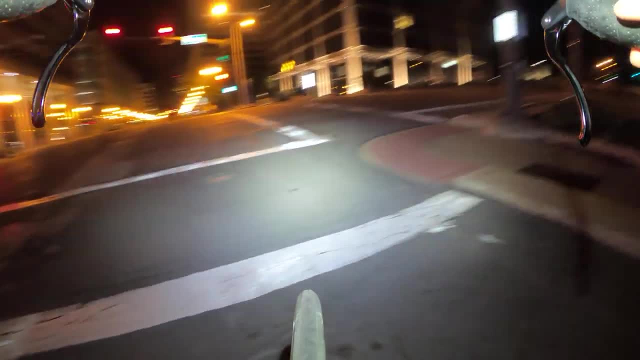 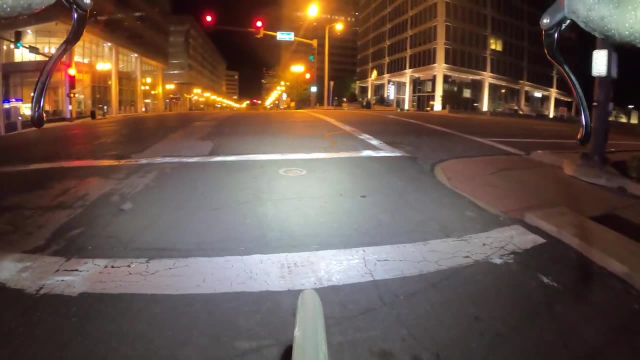 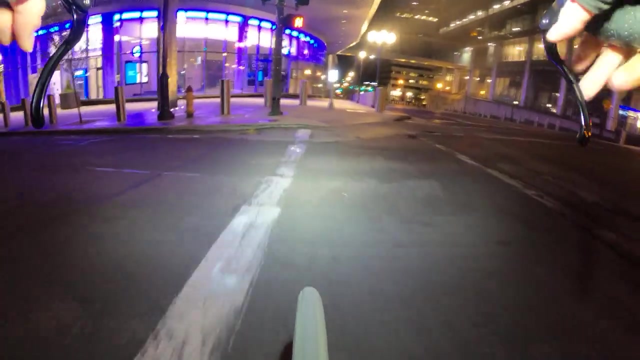 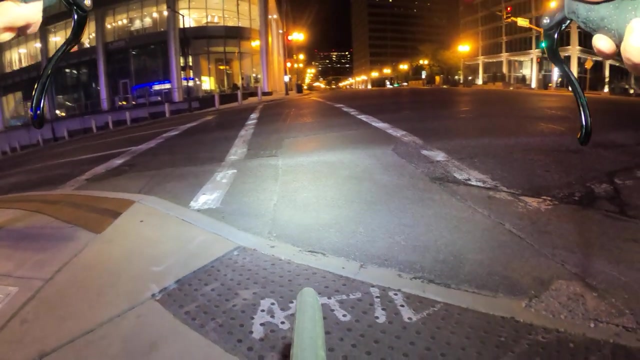 but, uh, sometimes you can try laying the bike down like this. see if you can, uh, get it to activate. there's nobody around. we're gonna go this way. see, it just went through a cycle. see, now it's like crosswalk here, so so we'll wait for the crosswalk, i guess. 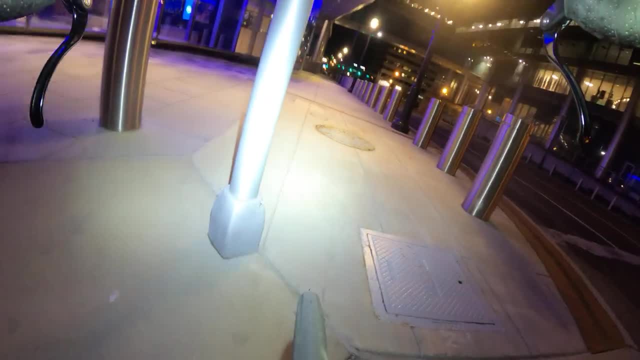 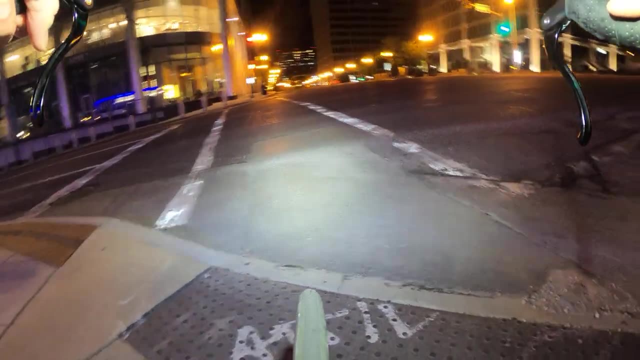 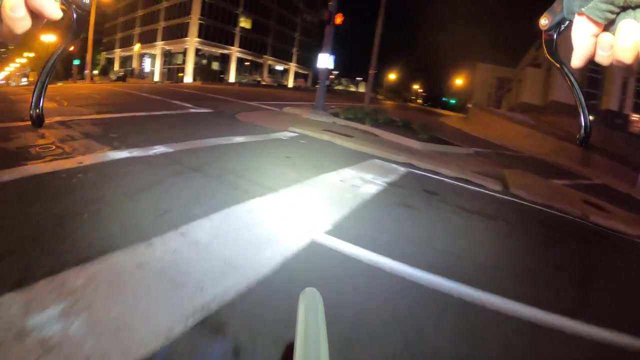 i can hit the crosswalk here. so now, since i hit the crosswalk which is going that way, i can scoot back out over here. usually i wouldn't actually go across there. i could hit the button right, could hit that button right there. i guess now that's changing the light for me. so there you go. 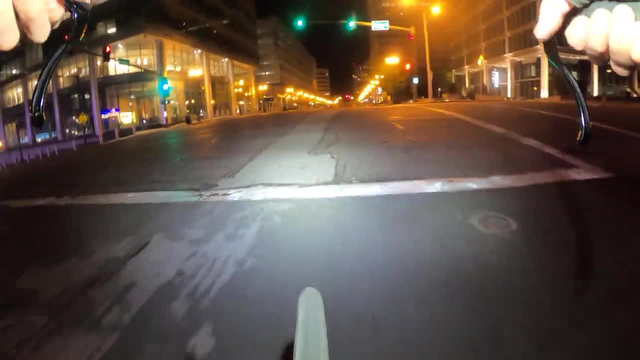 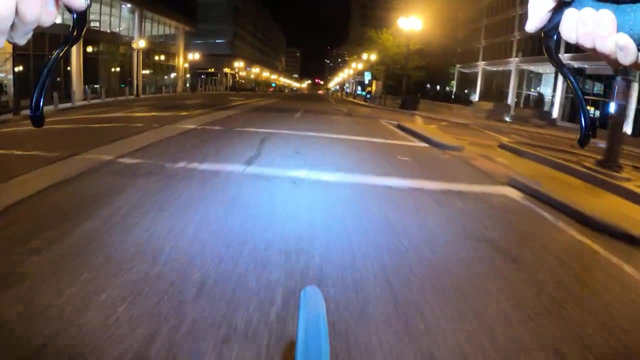 worst case scenario: you hit the crosswalk symbol. now i'll force the light to change and actually where i live, you're allowed to just go through the stoplight after you stop and there's no traffic around. uh, if it's gone through a cycle or two. 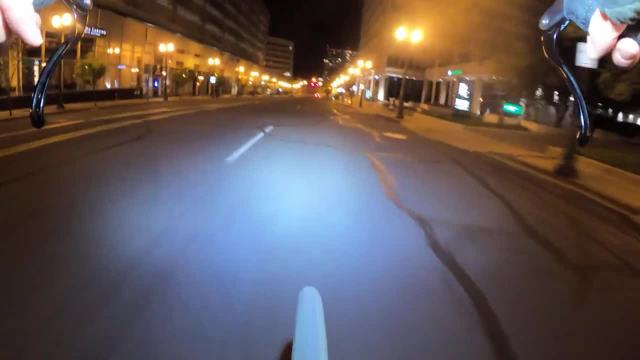 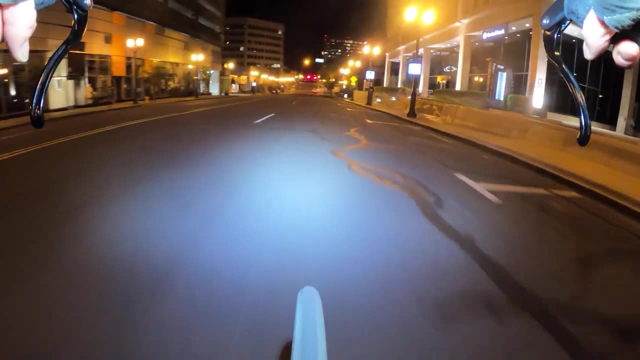 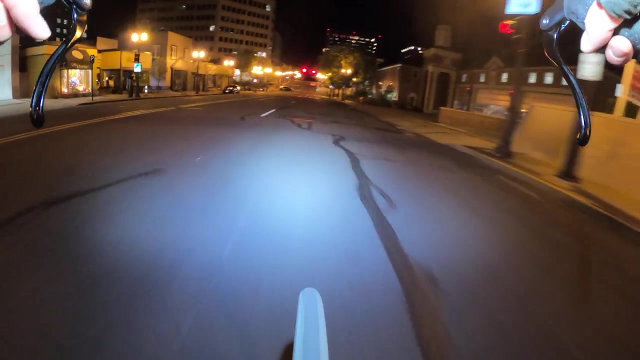 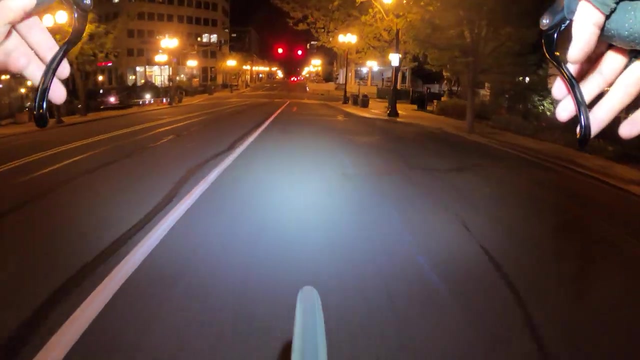 i have to look that up sometime, because i don't know exactly what the what the rule is for that. if it's like you gotta wait so many minutes or so many cycles for the light, i don't know. oh, it's windy, it is windy, so we're almost to work now. this has been tuesday morning. i'll see you next tomorrow day. 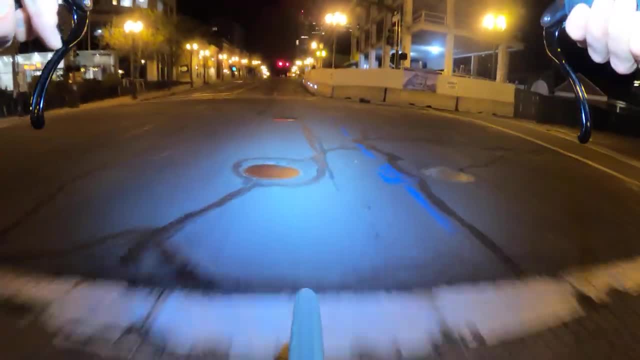 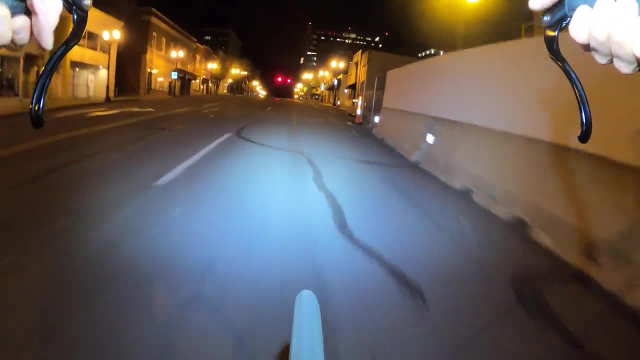 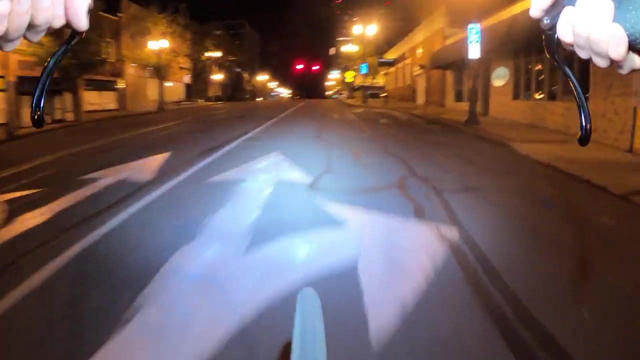 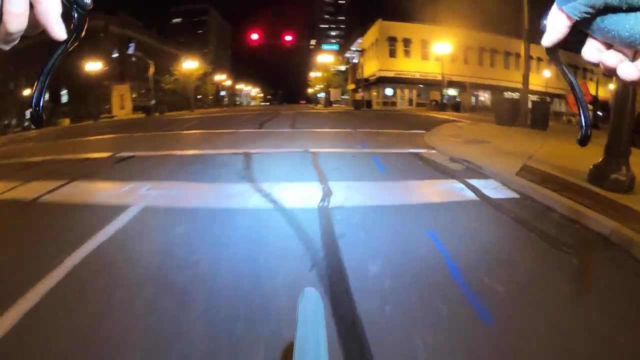 tomorrow, guy, wednesday, fuck the hell. if you have any other tips, leave them in the comment section below. i'm trying to hit all the kind of the basics here for bicycle commuting day by day here. so yesterday was plan out a route using a bicycle commuter. just google maps or whatever figure out, you don't check the street view. 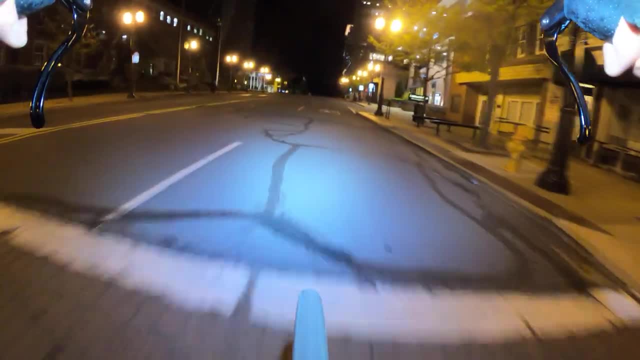 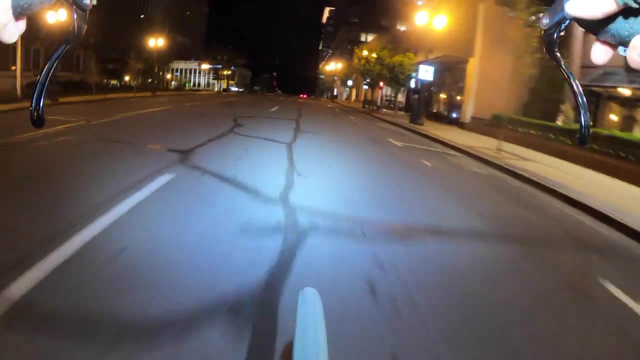 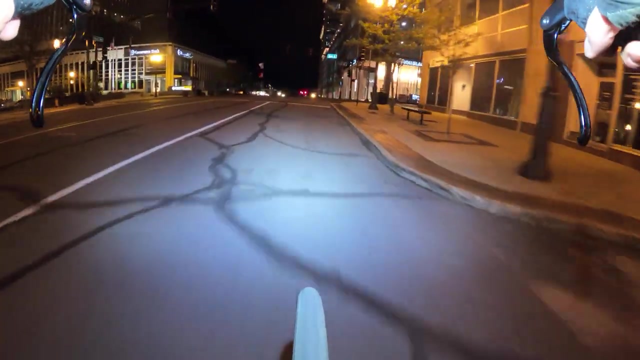 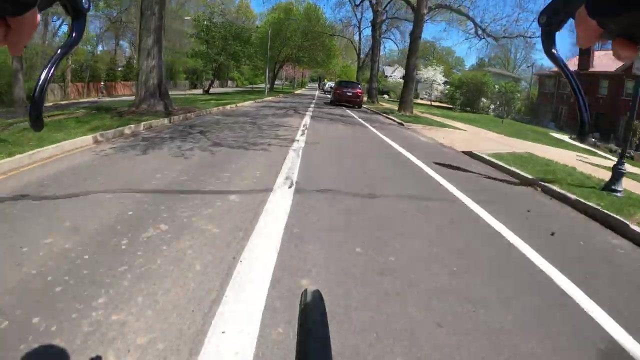 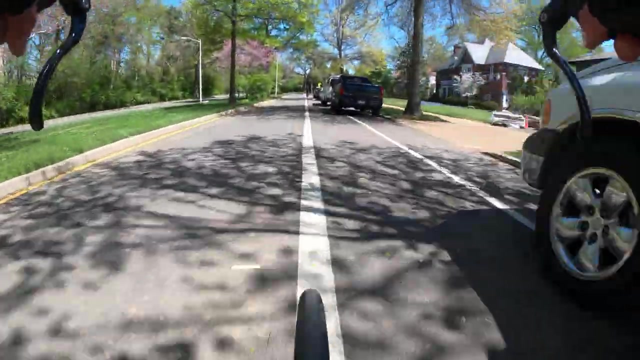 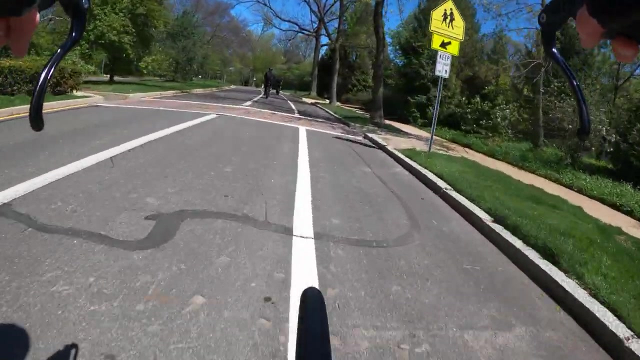 and today is, you know, kind of check the safety of your bike before you go. pump up those tires, pump up the tires, pump up the tires. see you next time, tomorrow, tomorrow, you, you.